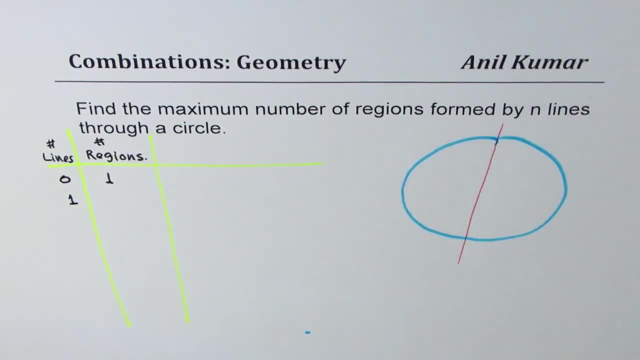 of like this somewhere. so we have two regions here, right? so what we have here is two regions. so let's rewrite these regions in a different way so that we can get a relation between the number of lines and the regions form. so, with no line at all, we have. 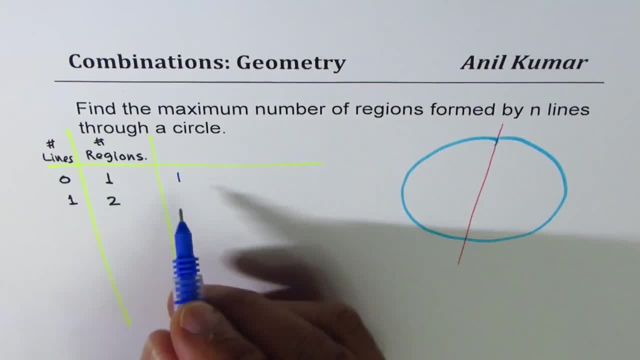 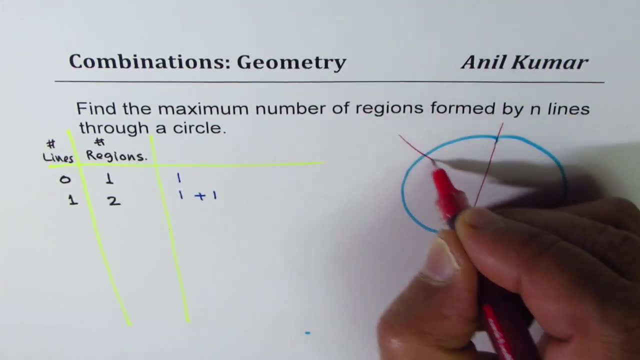 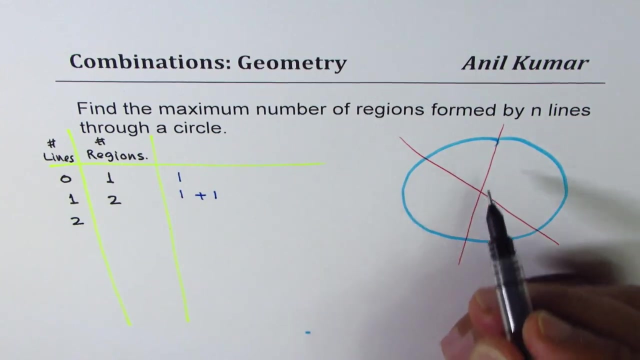 one region. as soon as we draw one line, we get two. that means one was already there, we added one more. perfect, now let's say we draw another line. so as you draw the next line, so we have two lines. now you can count. the regions are one, two, three, four. 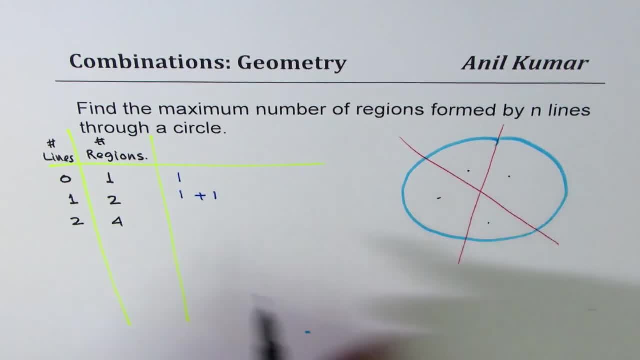 right. so these two lines added two more regions. so we could write this as one was there, without lines, and then we have one plus two, right? so one line gave one, two line gave two more. if I draw the third line, let us say, third line is kind of like this, so we can count the number of regions as one. 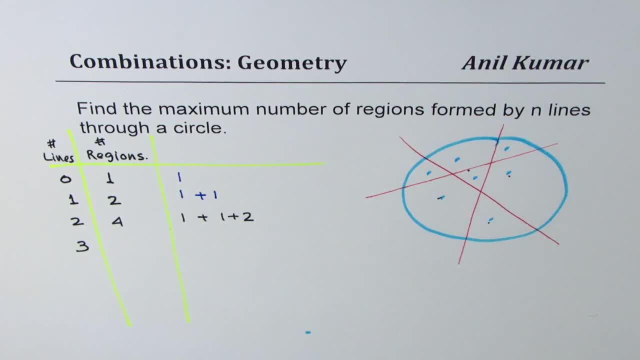 two, three, four, five, six and one, seven. so what we get here is seven regions. so we already had four, three more right, so we could write this as one plus one, plus two plus three. do you see that? so, if you observe, this particular pattern is kind of combination of the number of lines which we're drawing right. if I draw the fourth, 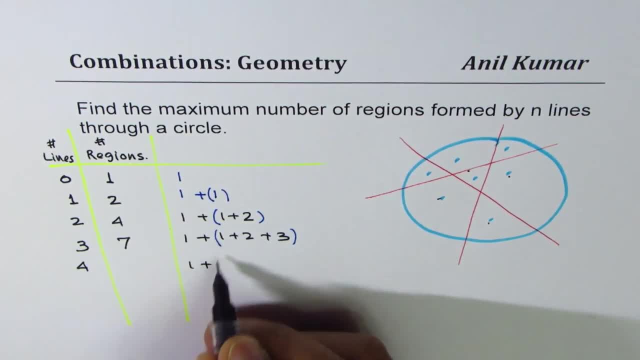 line, then what I expect here is one plus. we already have one plus two plus three. we expect four more regions to be created, seven plus four, 11 in all right. so that is how we can actually grow the number of regions: by increasing the number of lines. now, looking into this, if we go for n lines, then we expect this to be one plus two plus three.